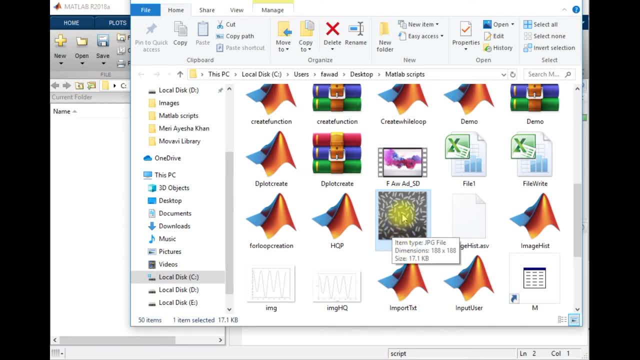 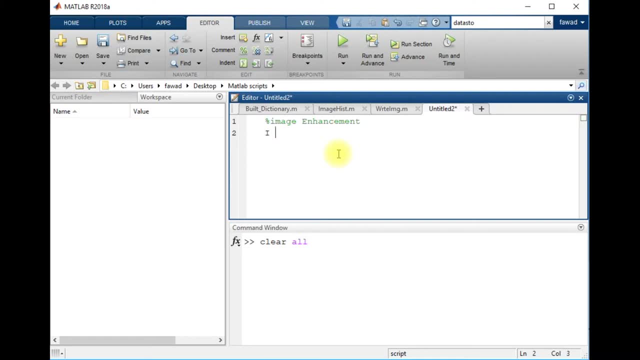 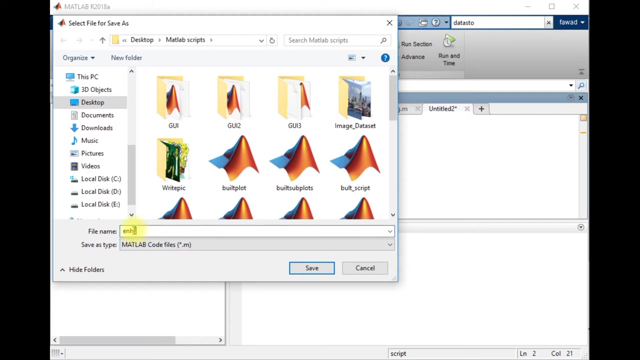 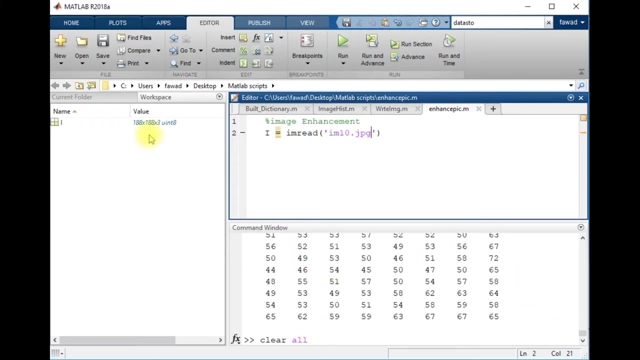 that is, the contrast is very low for this image. So now, uh, what I? I, how I am, how I will enhance this image. look at this, that I am going to read this image, im10.jpg. I will execute this and I see that I have loaded the image into MATLAB and this is the variable. 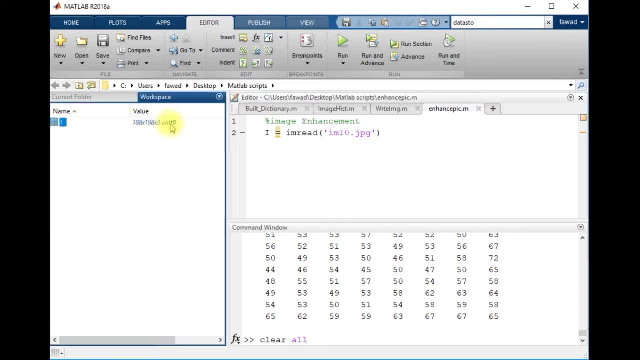 i. the dimension is 188.188.X3 and unsigned integer 8.. It is the data type of this image. I will read the image Now. let me display with it how this image looks like This one. I will use settestitier with the annotation value 184. the first option is: add image of this double row and the second option is add item query name. Now the person that you are using is red. Let me share it and see what this site does. So the This is the detailed image form image it will do Here. So there you go. I have see that I can increase this image. that is .188 frå 30 and. 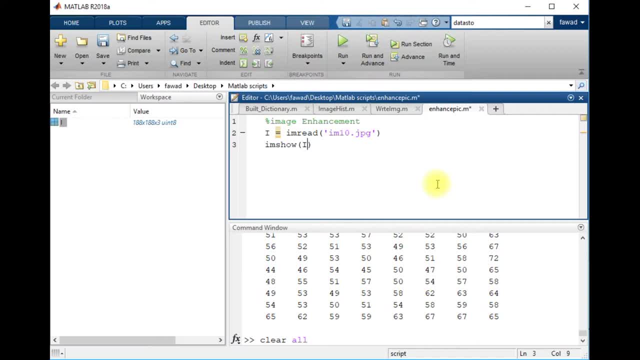 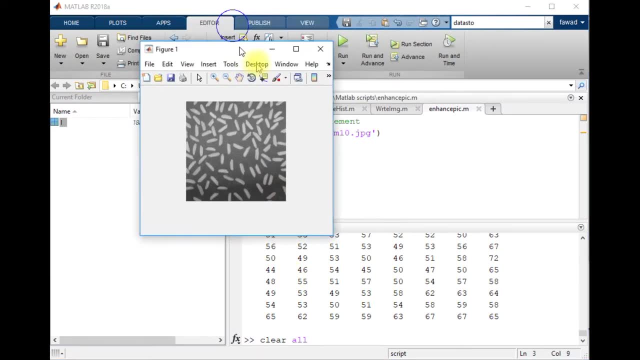 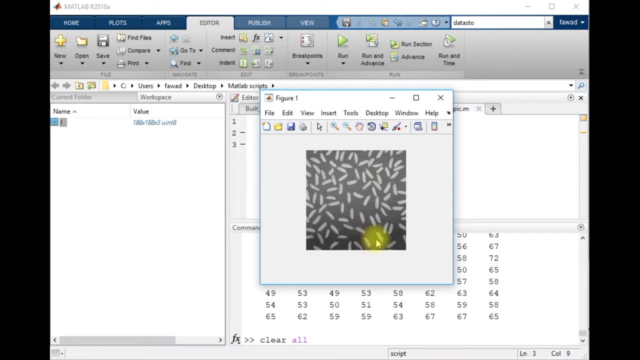 I am sure I now you can see that this is a very low contrast image and there are some noises like over here. you can see some spikes are here. so this is a image with some rice in. it is a texture created by rice on the table or some. 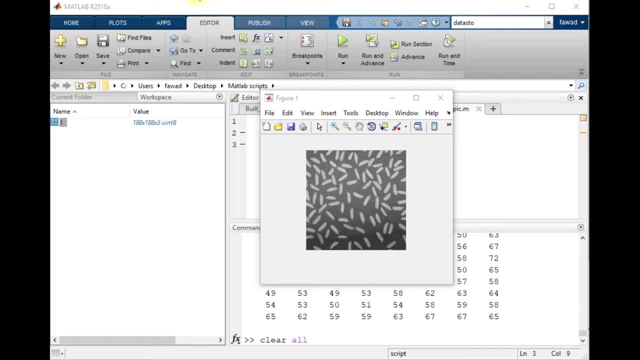 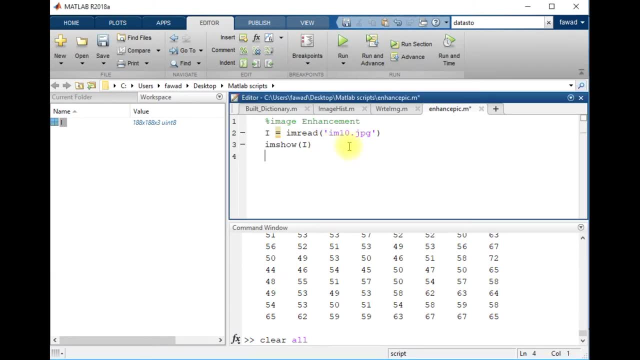 smooth surface. I am going to enhance this image in my lab. to enhance this image, I will have to predict the background of the image, like I will have to predict it how the background of this image look like. so, to find the background of this image, I will create a. 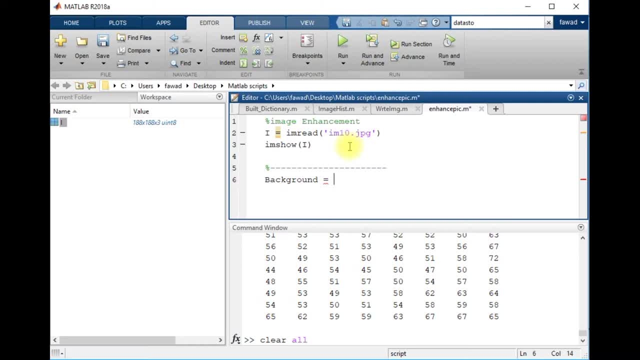 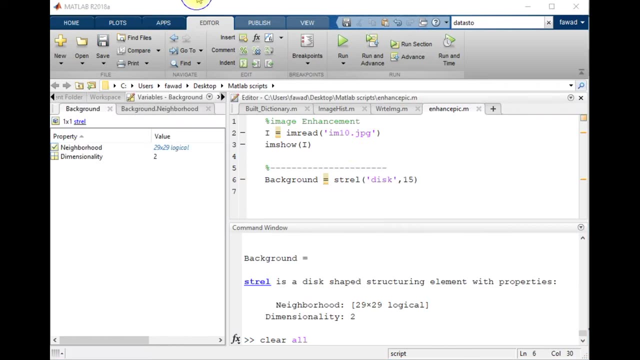 a disk. so I have created the background and you can see that I have created a disk of size 29 cross 29. but when I write a a disk of size 29 cross 29, but when I write a disk of size 29 cross 29, but when I write three over here and I execute the 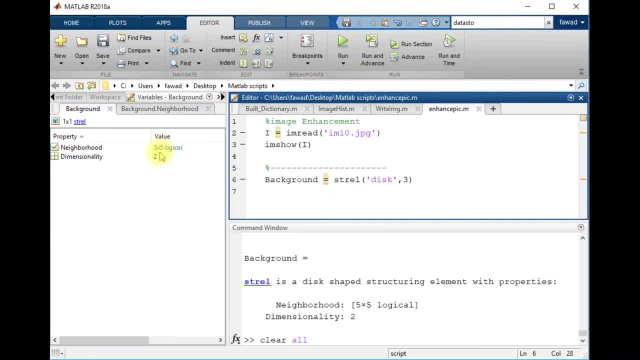 three over here and I execute the three over here and I execute the code: a disk size 5 cross 5 is created because code a disk size 5 cross 5 is created. because code a disk size 5 cross 5 is created because one pixel is the center and other. 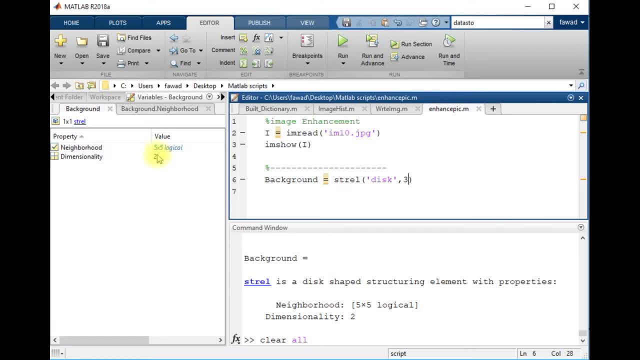 one pixel is the center and other one pixel is the center and other two are surrounding the center pixel. so the two are surrounding the center pixel. so the two are surrounding the center pixel. so the diameter is 5 cross 5, actually I want. diameter is 5 cross 5, actually I want. 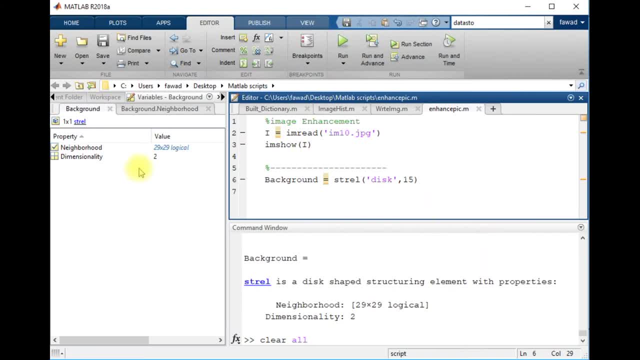 diameter is 5 cross 5. actually, I want to create a big disk, so I will create a. to create a big disk, so I will create a. to create a big disk, so I will create a size 5, 29 cross 29, so this is a 29 cross. 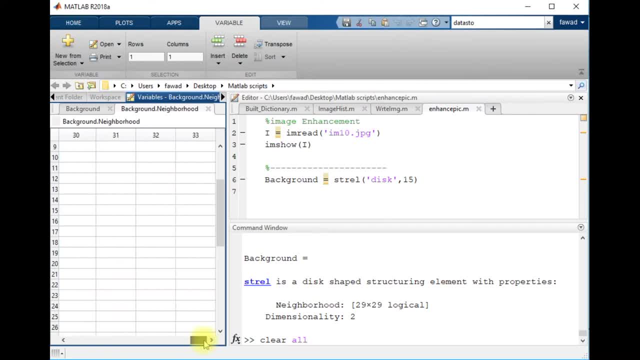 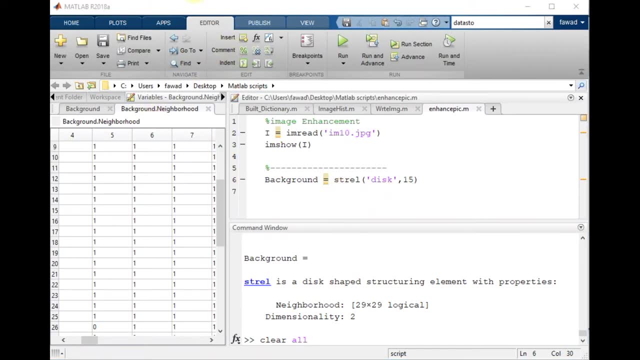 size 5: 29 cross 29, so this is a 29 cross size 5: 29 cross 29, so this is a 29 cross 29 discs. okay, now I will apply this 29 discs. okay, now, I will apply this 29 discs. okay, now I will apply this disc on the original predictive to. 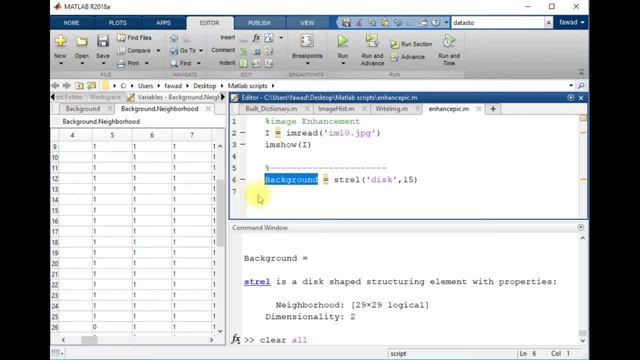 disc on the original predictive. to disc on the original predictive. to predict the background. I am going to predict the background. I am going to predict the background. I am going to apply the region opening operation. so apply the region opening operation. so apply the region opening operation. so this is the. I am open. 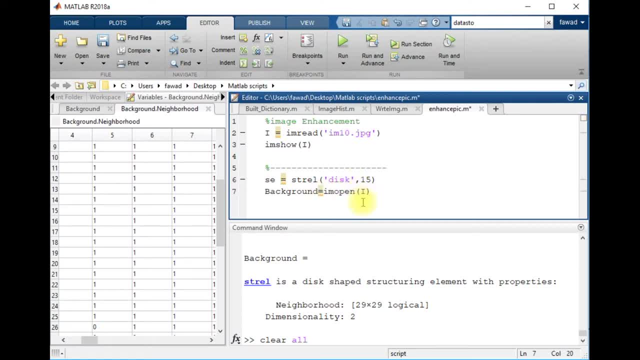 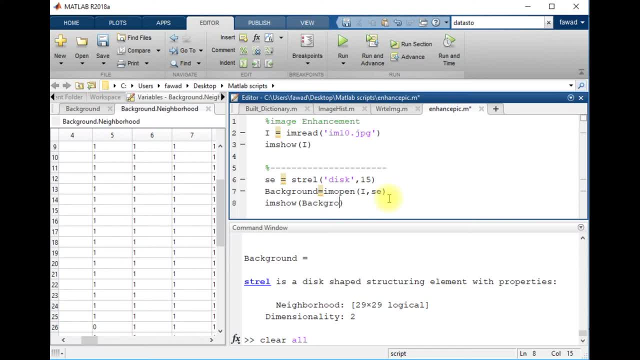 original image: I with SE and I am sure, original image. I with SE and I am sure ground subplot: two rows, two columns, ground subplot, two rows, two columns, ground subplot, two rows, two columns, and first in two rows, two column in the and first in two rows, two column in the. 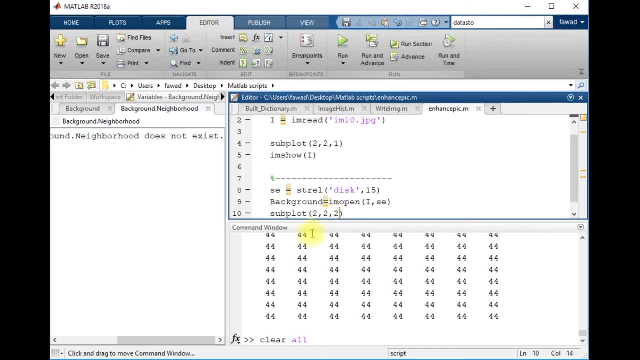 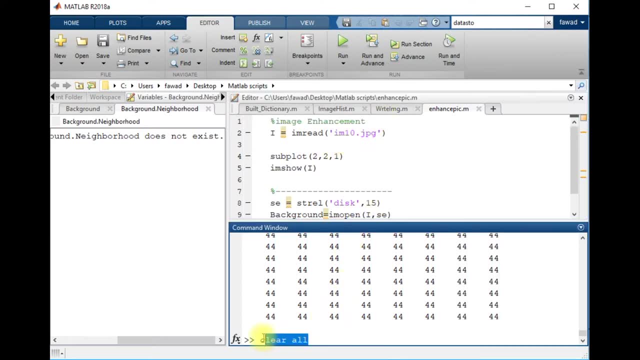 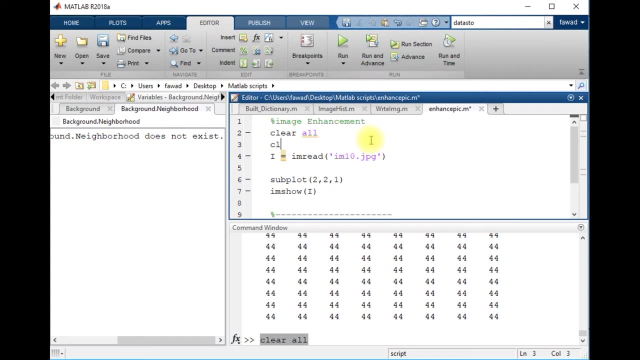 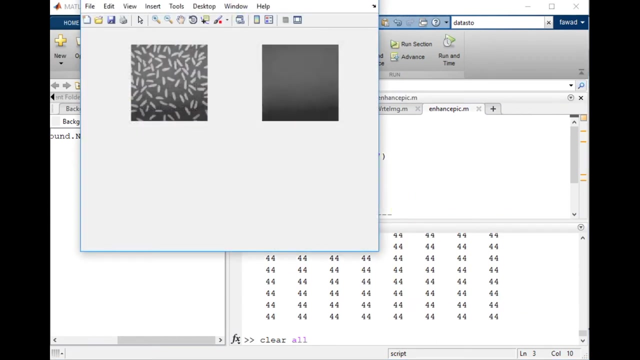 and first in two rows, two column in the second second. second: clear on, close on, clear on, close on, clear on, close on. so this is the image and this is the so this is the image and this is the so this is the image and this is the background. now I will subtract this. 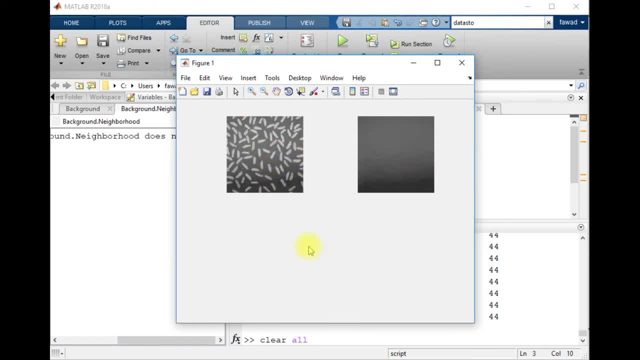 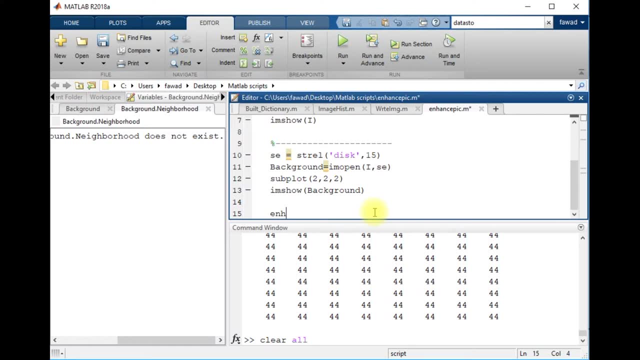 background. now I will subtract this background now. I will subtract this background from the original image and I background from the original image and I background from the original image and I will get an enhanced image. so in hands will get an enhanced image. so in hands will get an enhanced image. so in hands, enhanced image is equal to original image. 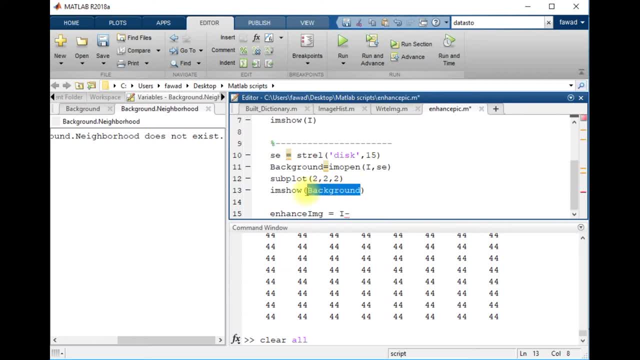 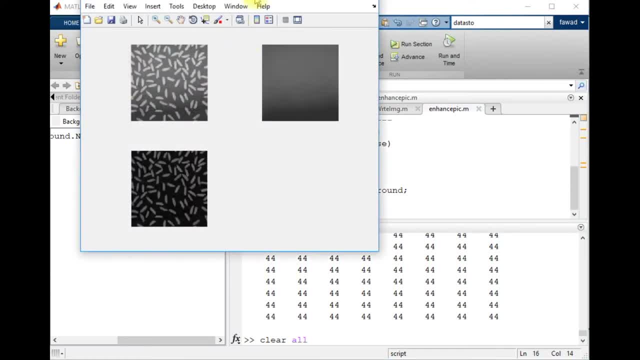 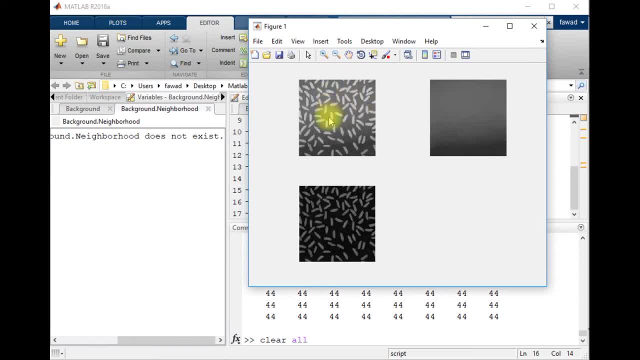 and when I display the enhanced image name of the enhanced images- enhance IMG- and I execute the code, I get this result. this was the blur image with the result. this was the blur image with the result. this was the blur image with the low contrast and this was the predicted. 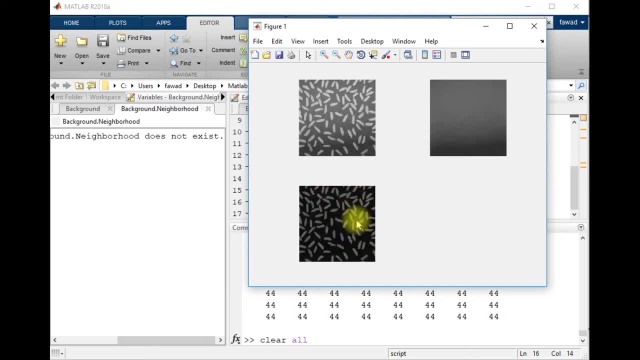 low contrast and this was the predicted low contrast and this was the predicted background. when we remove the background background, when we remove the background background, when we remove the background, we have got this type of result. so now I. we have got this type of result, so now I. 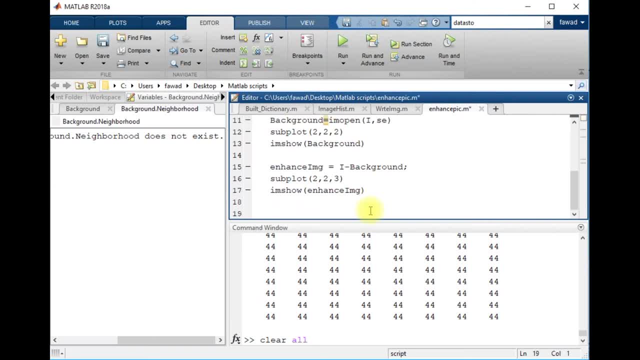 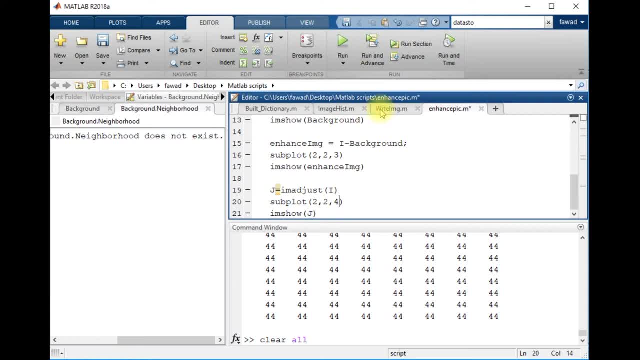 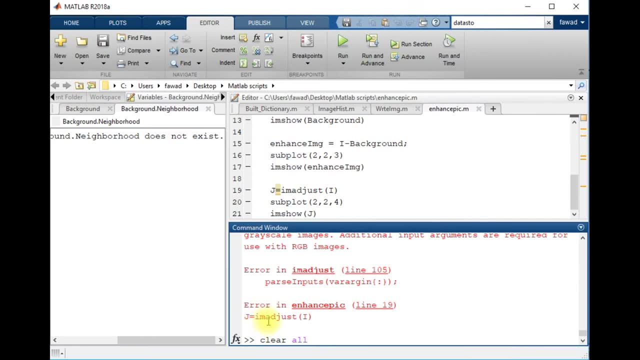 original. the J image content. the original. the J image content. the enhanced image now. enhanced image now. enhanced image now. okay, okay, okay, okay, okay. this is the same image, so I will display. this is the same image, so I will display. this is the same image, so I will display. is an error. 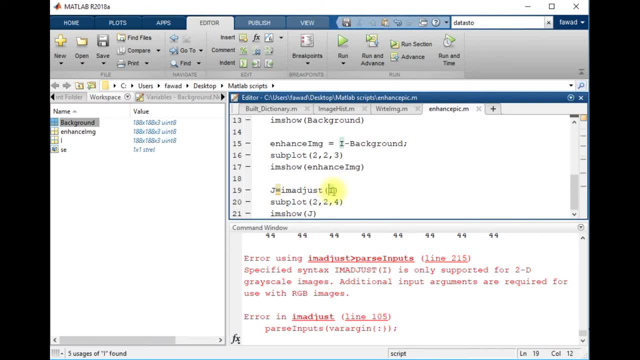 okay. it tell me the image would be okay. it tell me the image would be okay. it tell me the image would be grayscale. so I will apply RGB to gray to grayscale. so I will apply RGB to gray to grayscale. so I will apply RGB to gray to convert the image into grayscale before 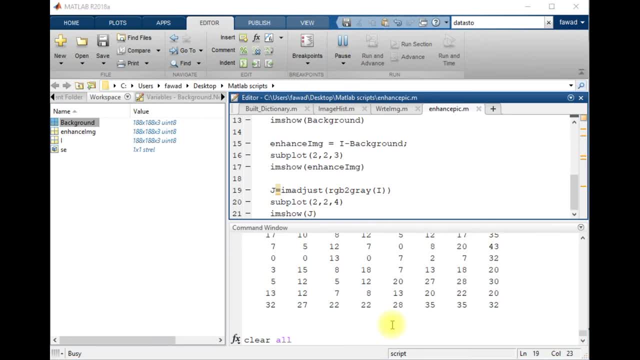 convert the image into grayscale. before convert the image into grayscale. before the execution of the code. now you can the execution of the code. now you can the execution of the code. now you can see there, this was the original image. see there, this was the original image. see there, this was the original image. is the background when we subtracted the. 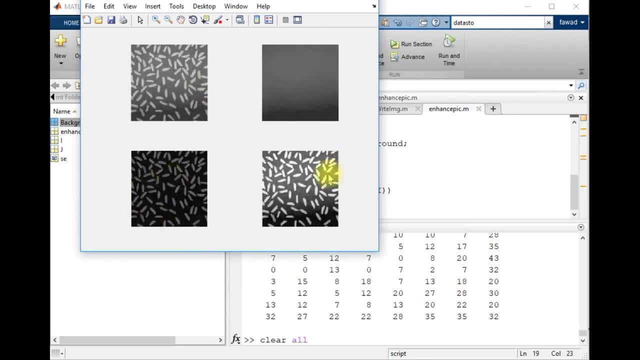 is the background when we subtracted the is the background when we subtracted the background from the image. we got this background from the image. we got this background from the image. we got this result after the contrast enhancement. we result after the contrast enhancement, we result after the contrast enhancement. we got this result. so this, there are many. 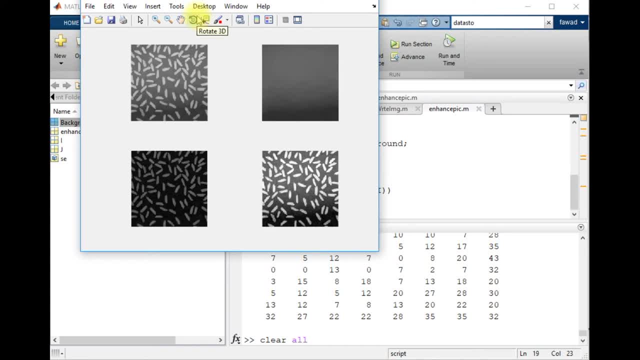 got this result, so this: there are many got this result, so this: there are many method to enhance the image in MATLAB. we method to enhance the image in MATLAB, we method to enhance the image in MATLAB. we can apply some more filters like we can. can apply some more filters like we can. 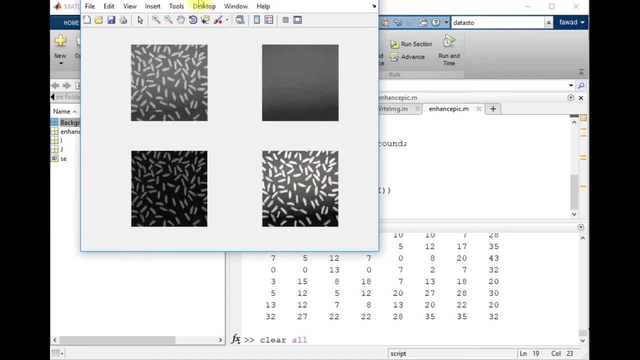 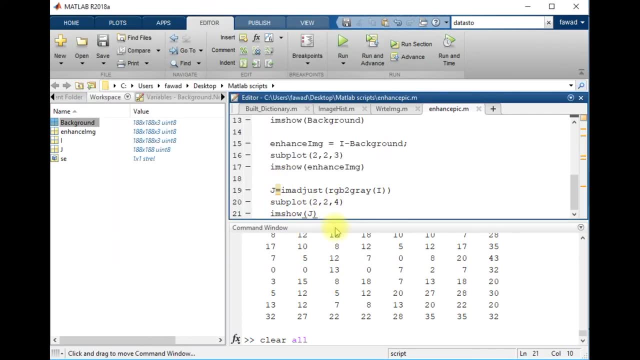 can apply some more filters, like we can remove some noises from the image. let me remove some noises from the image. let me remove some noises from the image. let me show you that- how you can remove some. show you that how you can remove some. show you that how you can remove some more noises from the image. so I will. 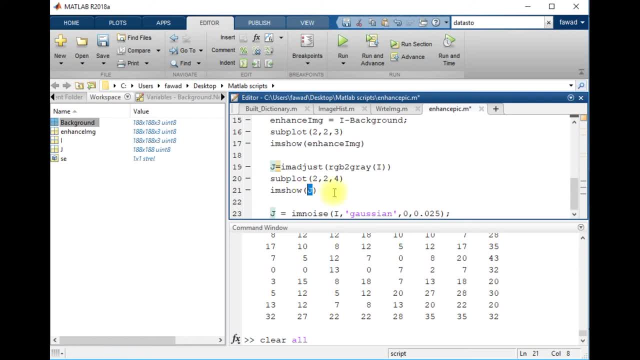 more noises from the image, so I will more noises from the image, so I will apply the Gaussian filter or the apply the Gaussian filter or the apply the Gaussian filter or the enhanced image. so this is the variance enhanced image. so this is the variance enhanced image. so this is the variance of the Gaussian filter. the shape of the. 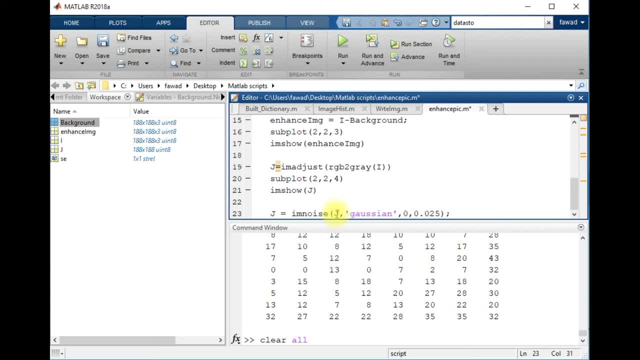 of the Gaussian filter. the shape of the of the Gaussian filter. the shape of the filter will be bell-shaped Gaussian and filter will be bell-shaped Gaussian and filter will be bell-shaped Gaussian. and we applied it will, we applied, it will, we applied, it will, J and we have got the image and I, J and. 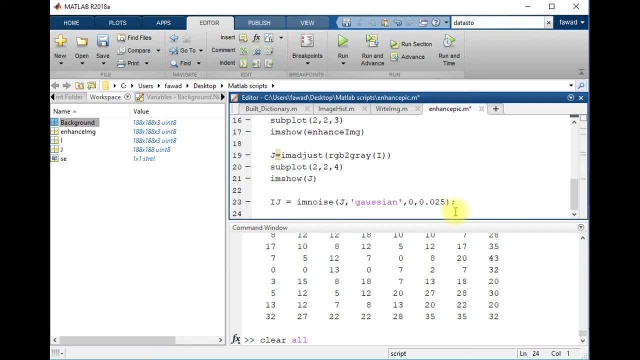 J and we have got the image and I J and J and we have got the image and I J and we will display this image to see what we will display this image to see what we will display this image to see what happened, happened, happened, happened, happened. 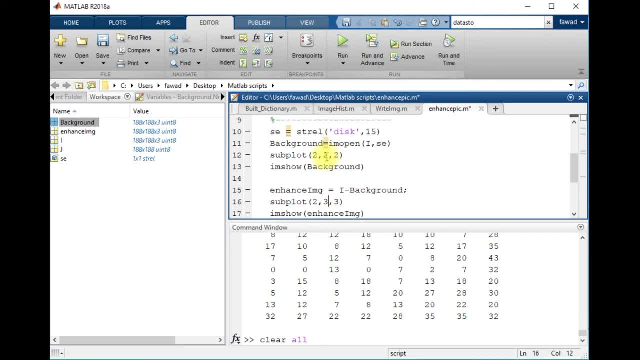 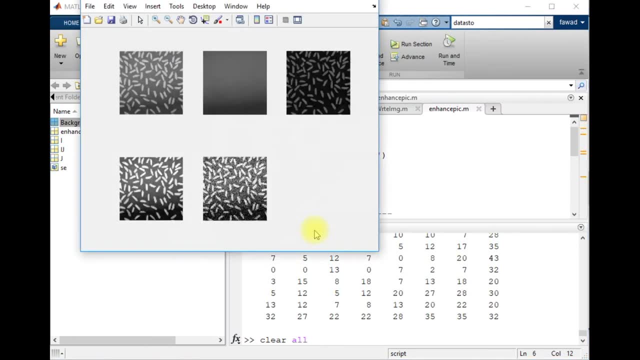 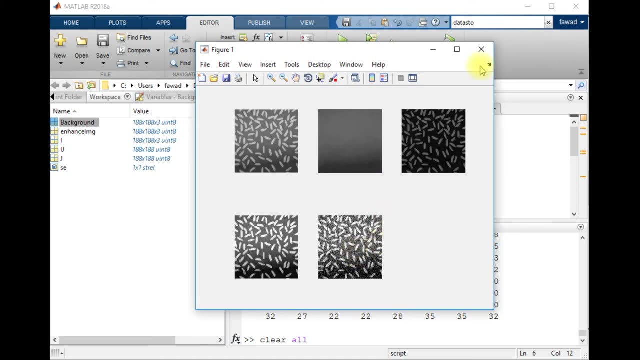 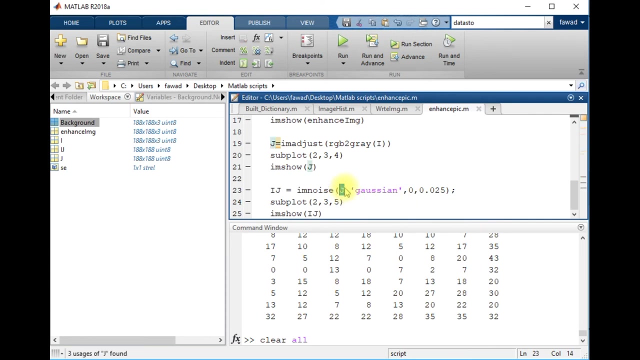 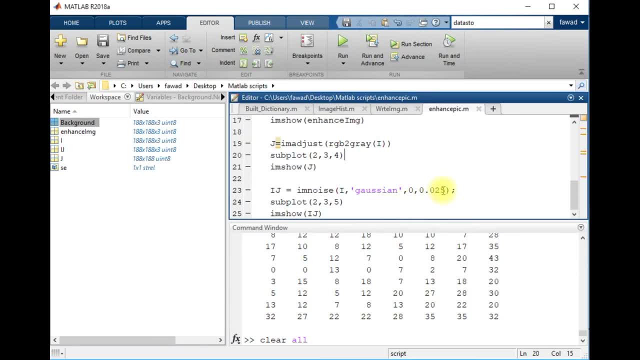 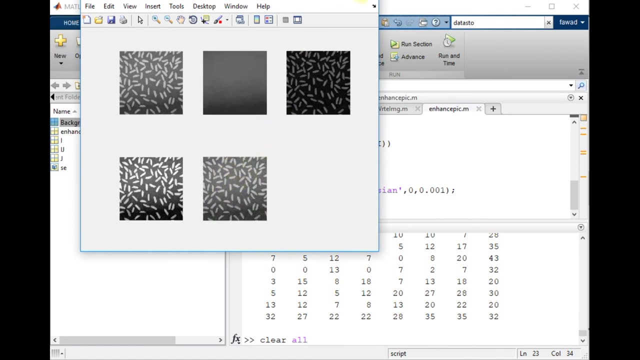 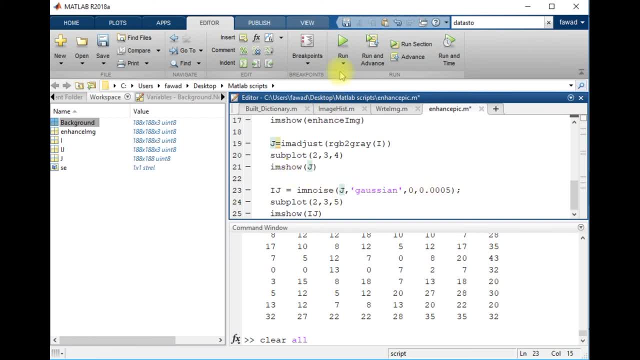 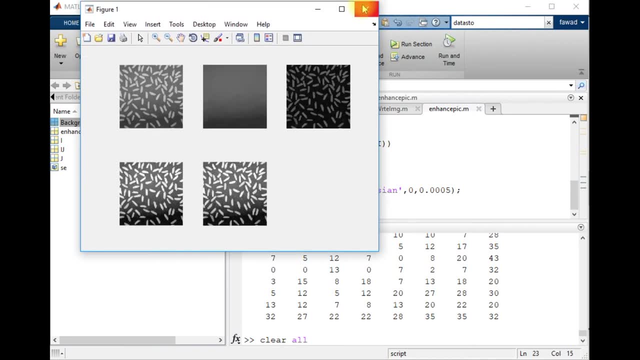 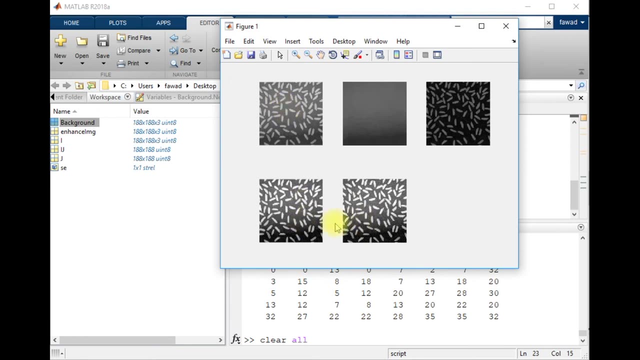 will apply it on the enhanced image. so this, there is a little improvement after applying the Gaussian filter on the enhanced image. there are many more filter that you can try. you can apply the date on the original image so you will get some more perfectly enhanced result of the original image, which was 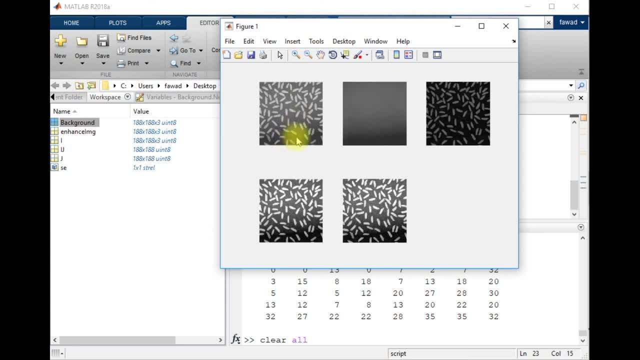 blur, which was hang, some noises which were having some variation in illumination, which was low contrast. so you can apply many more enhancement methods that are readily available in MATLAB, your functions, you can create even your own function in MATLAB because you know the logic that I have previously told you that how you can create logics in MATLAB. so thank you so much for being with us.